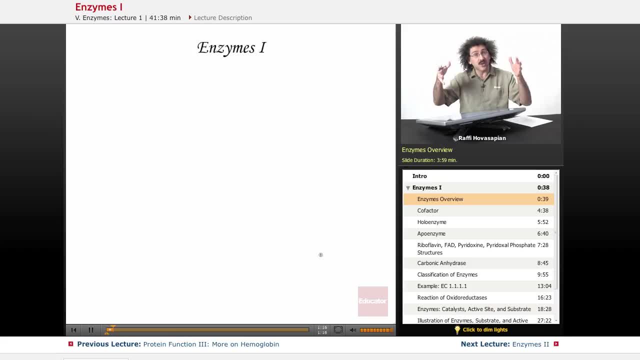 unnecessary. We just want to give you a good, solid grounding in enzymes And once we actually start to talk about the metabolic pathways- glycolysis, fatty acid breakdown, amino acids, amino acid breakdown, citric acid cycle, things like that- we'll be revisiting the enzymes. 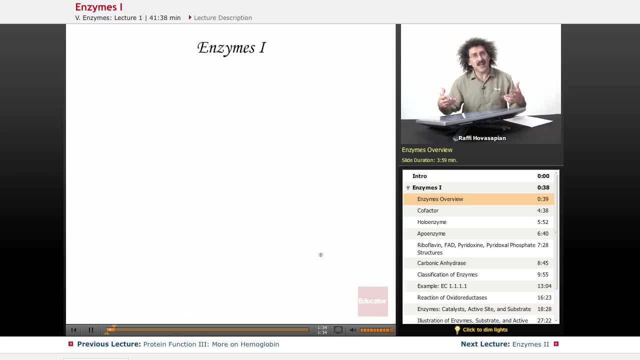 So a lot of what we ultimately want to learn about enzymes will come from all of the exposure that we get when we deal with the enzymes in the individual pathways. So, having said that, let's see what we can do. So enzymes are again, they are everything. So enzymes are proteins very 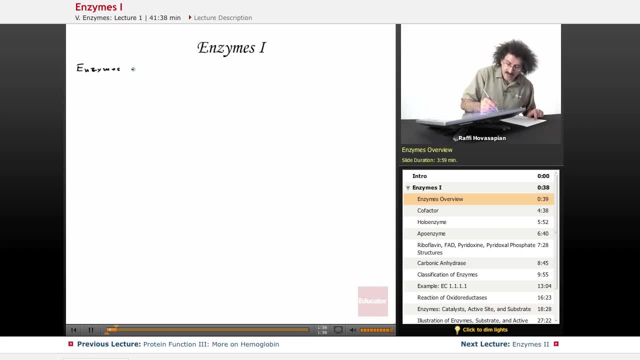 very large proteins. So enzymes are proteins, very, very large proteins. So enzymes are proteins, proteins. So enzymes are proteins, proteins. The only exception. exception are the catalytic RNAs, the RNAs which you'll end up discussing in a subsequent class, molecular biology. 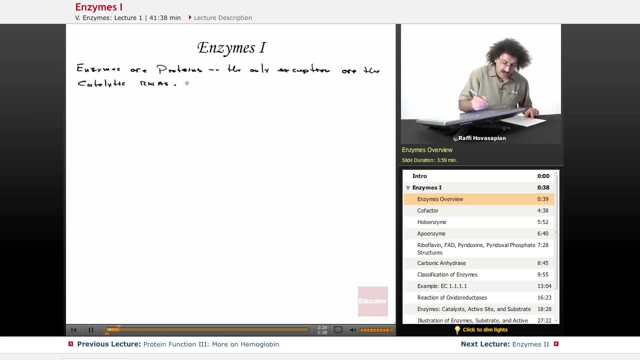 Catalytic RNAs. Okay Now, some enzymes function as is. Some enzymes function as is, That is, without additional chemical groups to help them along, So without additional An desde la búsqueda de química chemical groups to make them work. 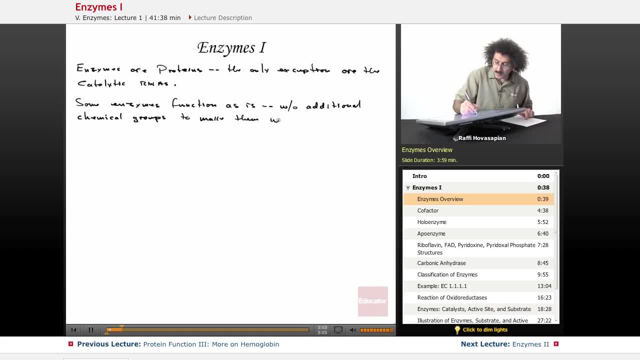 Consecúca. other enzymes function as is. Others require something called a cofactor, So let's get comfortable here. So others, consecúca until consecúca. other enzymes function as is, So this is something called a cofactor. but let's look at the different functions of an enzyme. 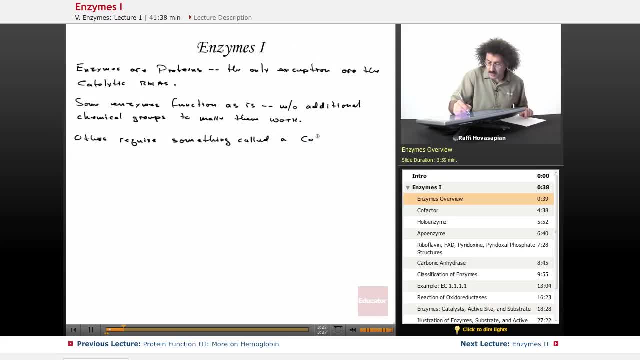 so let's look at the different functions of an enzyme, something called a cofactor. So a cofactor can be one of several things. It can be an inorganic ion, you know, maybe like iron 2+, or maybe magnesium 2+ or manganese 2+, etc. zinc. 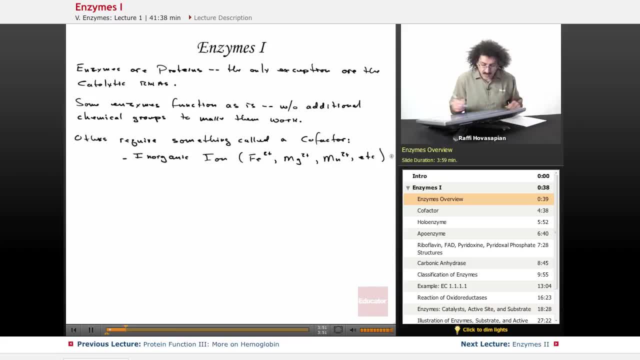 cobalt, something like that. It can also be an organic molecule, an organic or occasionally a metalloorganic molecule called a. we usually call it a coenzyme because it is an actual molecule, it's not just one single metal ion called a coenzyme. 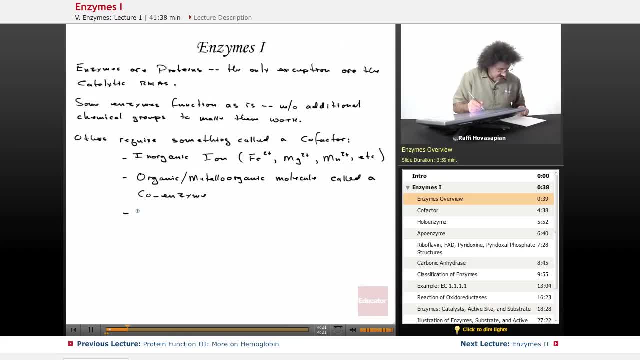 Coenzyme. Now, some enzymes require both, both ions and coenzymes. Okay, now when an ion or you know what, let's just call it a cofactor. Okay, all these names that we're throwing around, I know it can tend to be a little bit confusing. 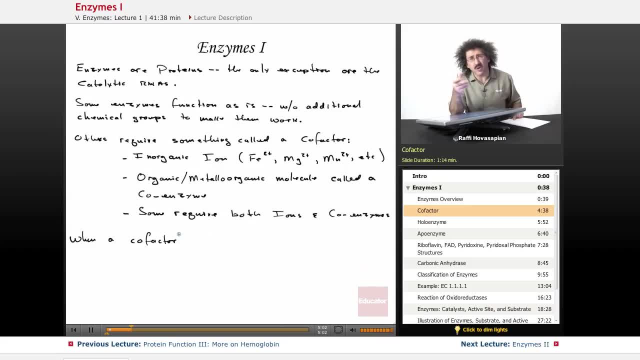 The names themselves are not altogether that important, except for the occasional quizzes that you take. What's important again is the chemistry, just understanding what the function of these things is. So when a cofactor, either ion or coenzyme, is tightly, 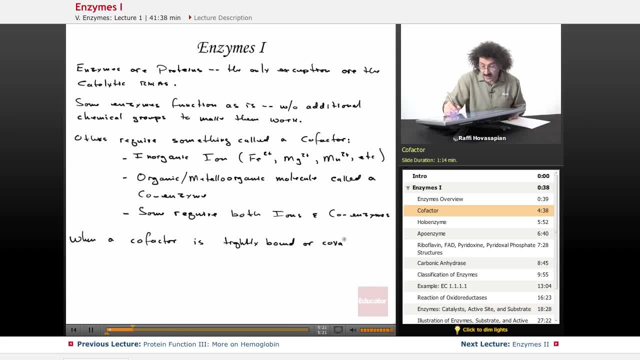 bound or covalently attached. covalently attached to the enzyme, we usually call it a prosthetic group. Now let's see the entire. let's try this again. enzyme plus cofactor is called a holoenzyme. Again, just a bunch of nomenclature. that's not altogether that. important. So when you have the enzyme plus its cofactor, the thing that's all ready to go, it's called a holoenzyme. The enzyme part alone, without its cofactor, it's called an apoenzyme Enzyme. 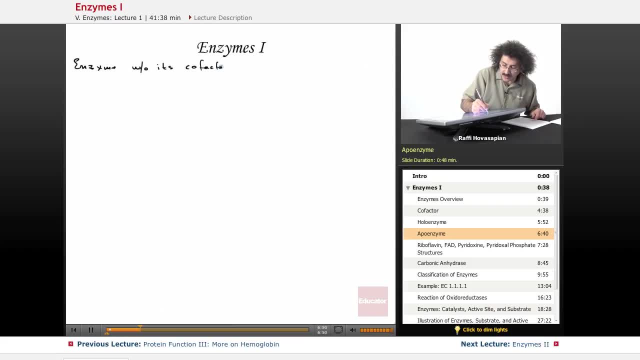 without its cofactor is called an apoenzyme, or sometimes an apoprotein. Okay, Now, most coenzymes coenzymes. they derive from vitamins. Okay, So some examples would be well, let's actually take a look at some. So we have this one right. 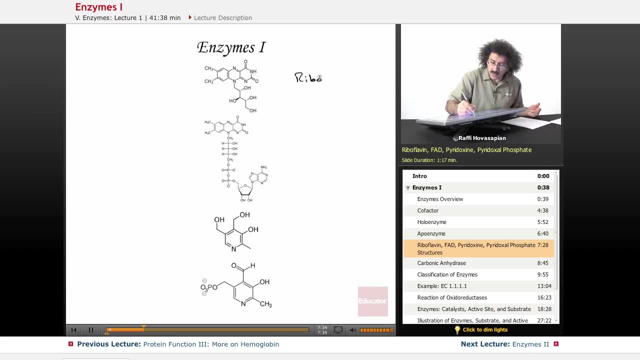 here, This first one. this is riboflavin. Okay, This is one of the vitamins that we need to ingest in order for bodies to function properly, And the enzyme that is derived from riboflavin. this part right here. you notice, it's right here. 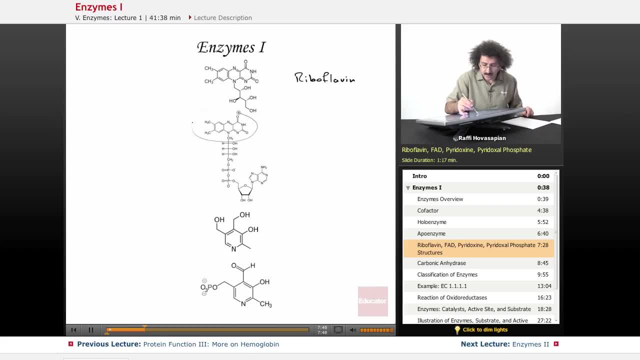 Okay, This is right here. Okay, This is this. looks like flabenedenine dinucleotide. That is the coenzyme form of the riboflavin. We ingest the riboflavin, the body converts it to FAD. 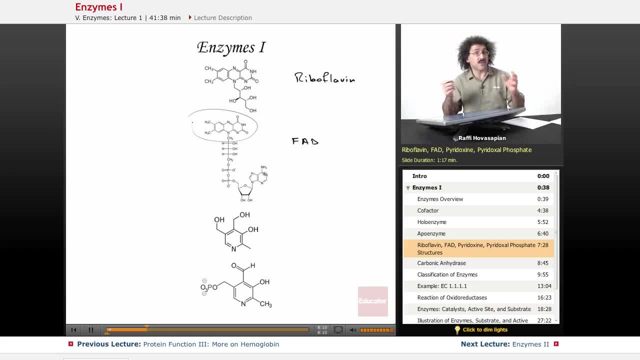 This is the coenzyme, This is the active part that works in concert with the particular enzyme that it's attached to. Okay, Another one would be. another vitamin would be pyridoxine, And pyridoxine is the vitamin that we ingest. 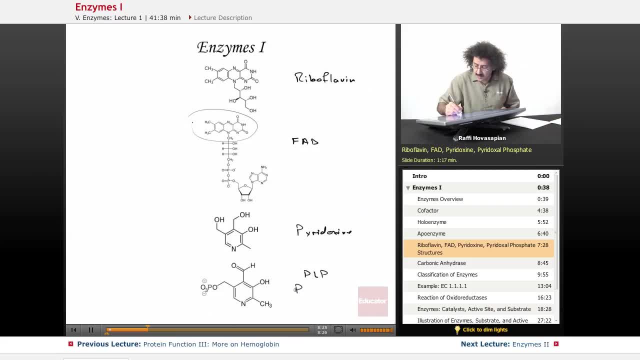 The coenzyme itself is something called PLP. It's called pyridoxal phosphate, pyridoxal phosphate, And again, we'll be running into these. We'll be getting into more details later on When we speak about specific enzymes. 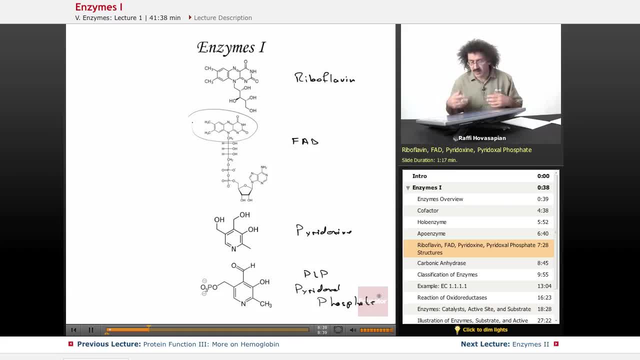 we're going to talk about these cofactors, what they do, how they do it. We're going to get into detailed mechanisms and things like that Right now. just wanted you to see some examples. Let's see a couple of other examples. 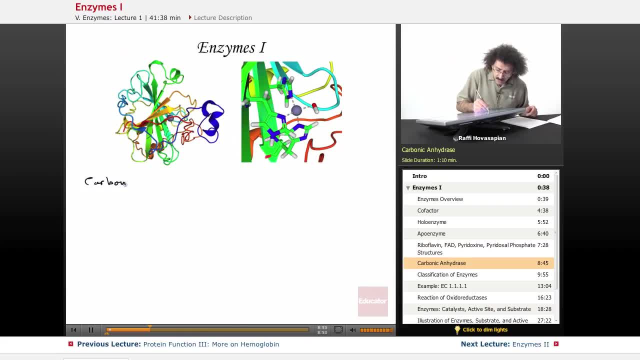 We have carbonic anhydrase, So just wanted you to see, actually in this case, a ribbon diagram of the actual enzyme itself And I don't know if you can see it here- that little zinc ion. So that is a prosthetic group for. 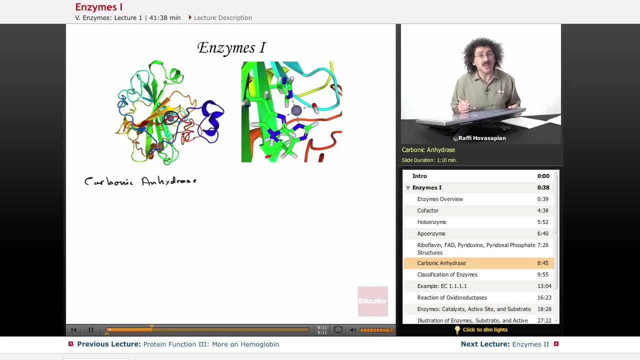 it's a cofactor for carbonic anhydrase, Happens to just be a metallic ion And this, of course, is a close-up view. This is zinc ion. You see, it's coordinated to a histidine, to another histidine. 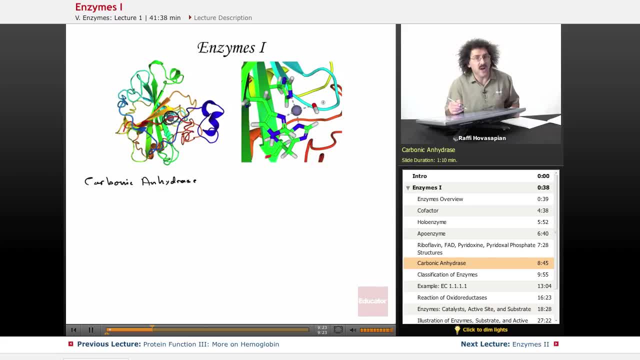 to another histidine And it's also coordinated to a hydroxide ion. So within the enzyme, within the folds of the enzyme itself, there is this what you might call a partial active site. This particular zinc ion is coordinated to three histidine residues and a hydroxide. 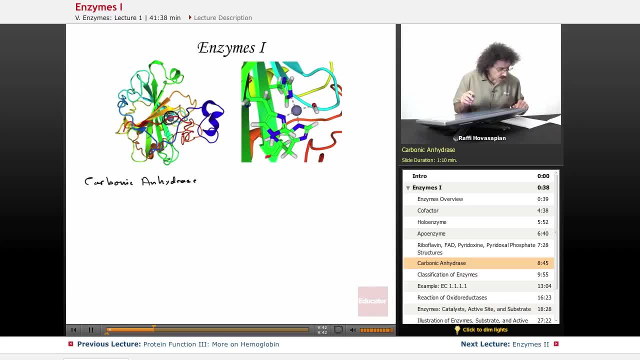 That's it. Nothing particularly strange going on here. OK, So now I'll just write close-up here, Close-up of the carbonic anhydrase. OK Now, enzymes are classified according to the reactions they catalyze. That makes sense. 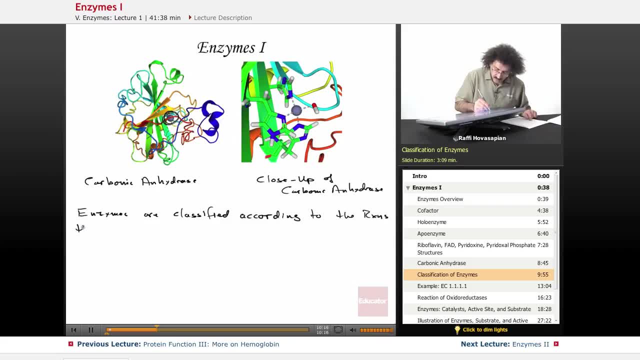 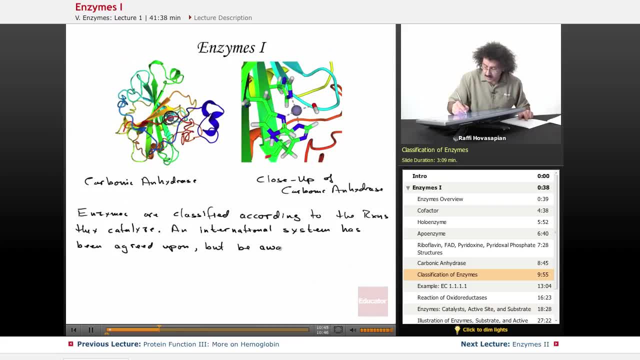 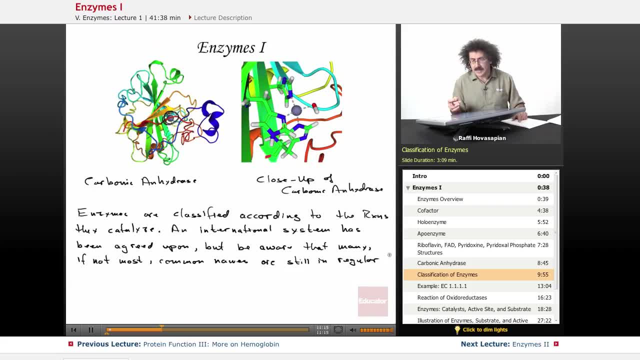 Agreed upon. Agreed upon. we'll be referring to things with their common names. We'll be calling them, for example, alcohol dehydrogenase. We won't be calling it alcohol NAD oxidoreductase. That's going to be the formal name. 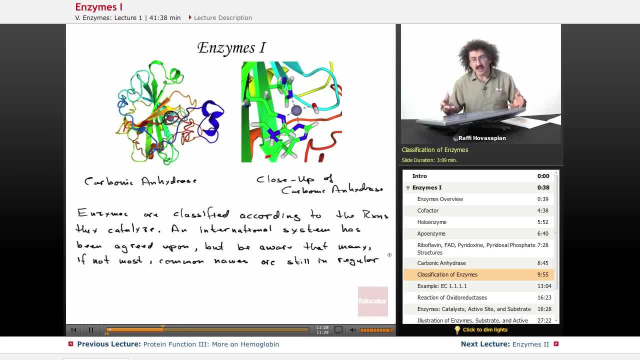 For the most part, we're going to be using common names. Now, clearly, a lot of the enzymes that were discovered early on before the International Agreement of Systematization, those common names I mean, they're just so entrenched in the literature. 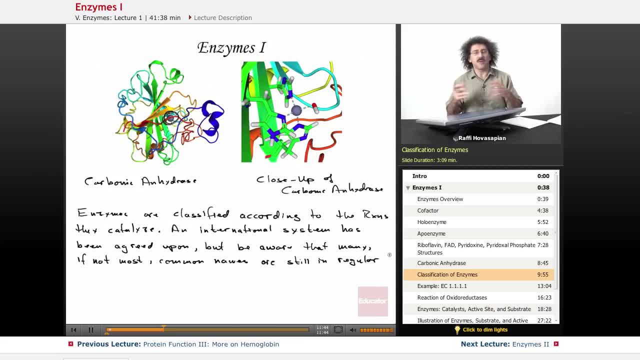 They're just so entrenched in our daily use that they're never going to go anywhere. So they have formal names, but it's the common names that you're going to see them as The more recently discovered enzymes. those are the ones where you're going to actually use the systematic name. 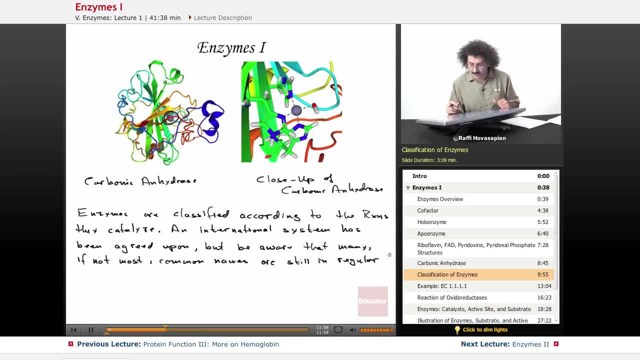 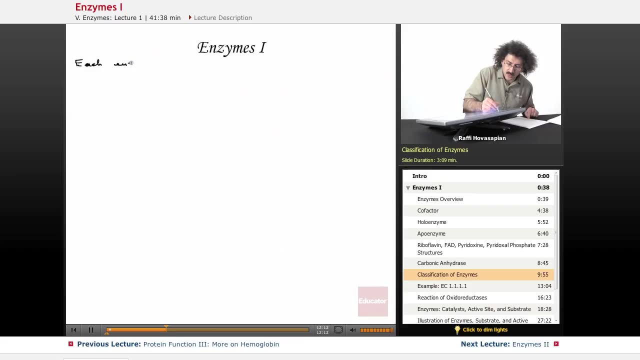 instead of the common name, because no common name exists for them. Okay, so, common names are still in regular use. So let's see here, Let's go ahead and move on to this. So each enzyme, So each new enzyme, or each enzyme. 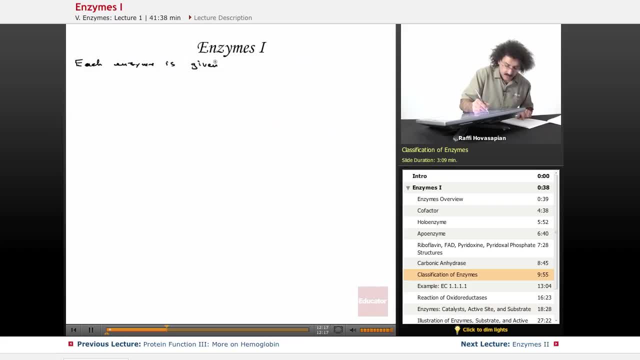 Enzyme is given a number. It's called the enzyme commission number- Enzyme commission number and a systematic name. So it's given both a number And a name. Now the EC number has four digits. The first number specifies the class of the enzyme. 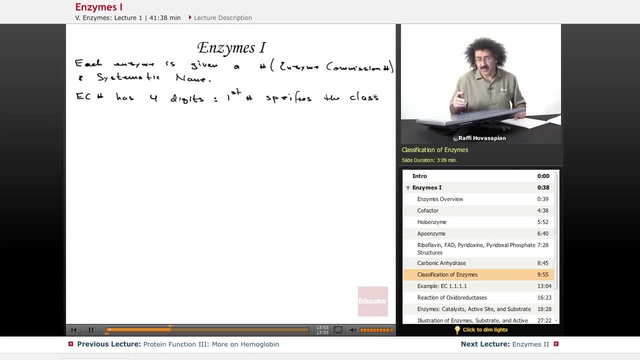 Specifies the class, the enzyme class. There are six classes, So an example would be: And then of course, you have your subclasses Underneath that. an example would be: let's just take the most basic one: EC 1.1.1.1. 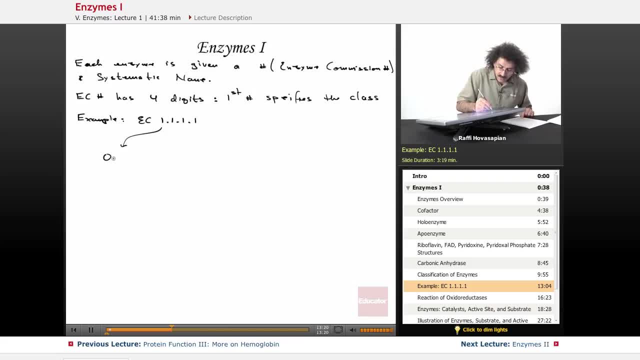 So class one. these are enzymes and they are called oxidoreductases. They are involved in electron transfer, Oxidation reduction. They're involved in electron transfer, facilitating the transfer of electrons From one molecule, From one molecule to another molecule. 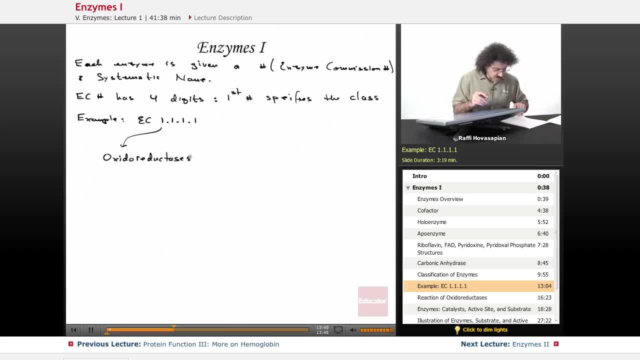 From one substrate to another substrate. The transfer of electrons, Transfer of electrons. So that's it, That first number, that's what that specifies. So let's go ahead and look at a systematic name. So in this particular case, the EC 1.1.1.1.. 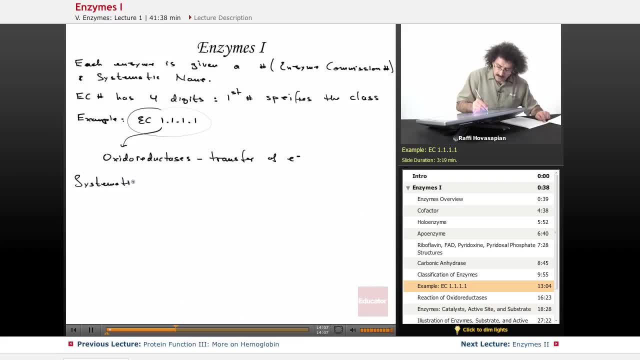 It's systematic name. It's going to be, as we said, alcohol, colon NAD plus oxidoreductase. Oxidoreductase tells me there's a transfer of electrons. alcohol electrons are transferred from the alcohol. 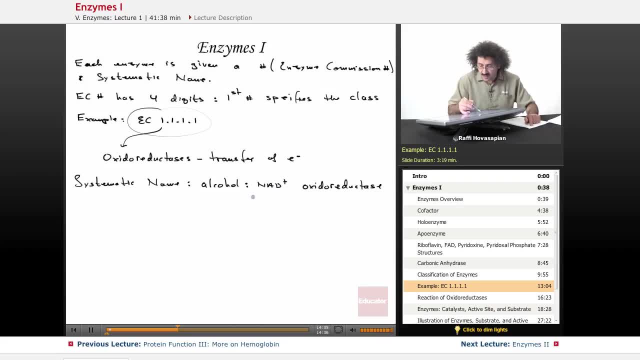 There's a colon, They're transferred to NAD plus. That's what this means From here to here: Oxidoreductase- The common name. common name is alcohol dehydrogenase, Alcohol dehydrogenase. This is the enzyme that's responsible for metabolizing the alcohol that you drink. 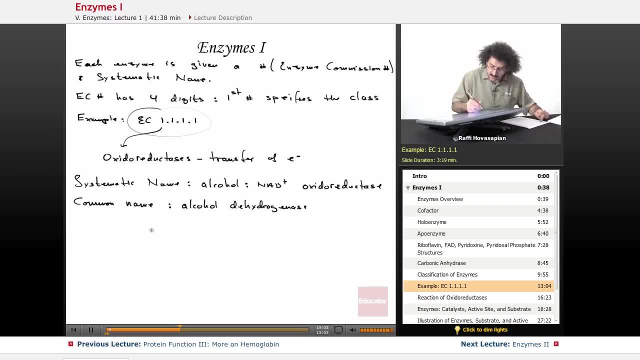 So it doesn't poison you. Alcohol dehydrogenase. Okay, So now we have the 1.1.1.1.. This: This: This is the. this tells me that it's class an oxidoreductase. 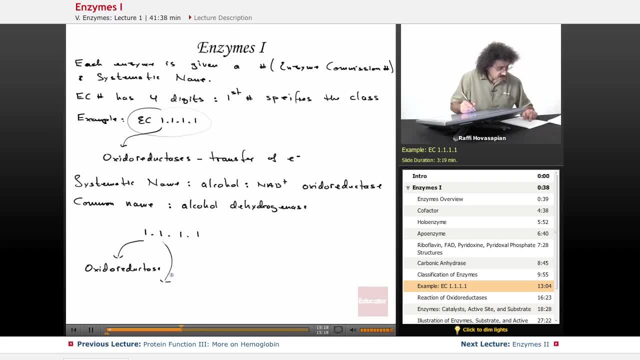 Okay, This one right here. it tells me that it's acting on an alcohol group, a COH group. This one right here. the third number: it tells me that the electron acceptor is either NAD plus or NADP plus. 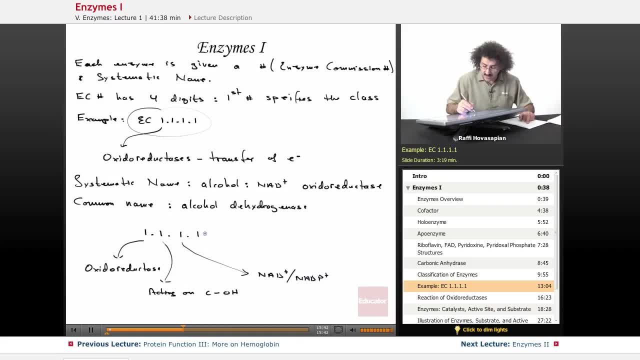 And this one right here. it's specifically NAD plus. If you had 1.1.1.2, that would be alcohol dehydrogenase, NADP plus. That's it. So, really, what's I mean ultimately? what's important I mean are all of the numbers. 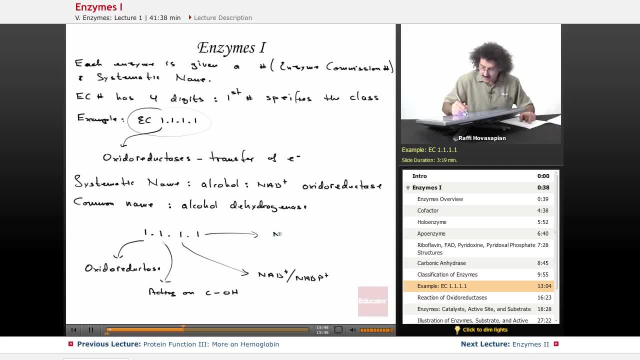 I mean, you can look all of these up, It's not a problem. You don't have to know any of these. It's really important to know that the first one is NADP plus. The second one is NADP plus. 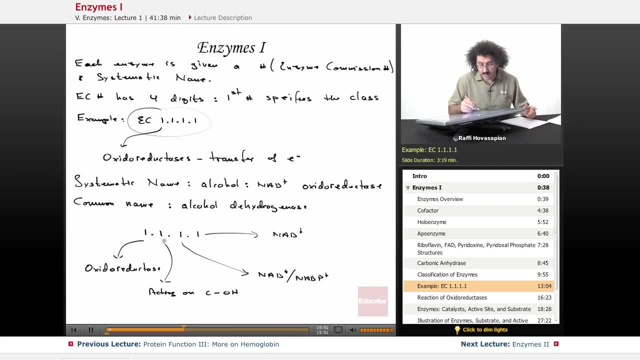 The third one is NADP plus, The fourth one is NADP plus. The fifth one is NADP plus. The sixth one is NADP plus. The fifth one is NADP plus. The sixth one is NADP plus. 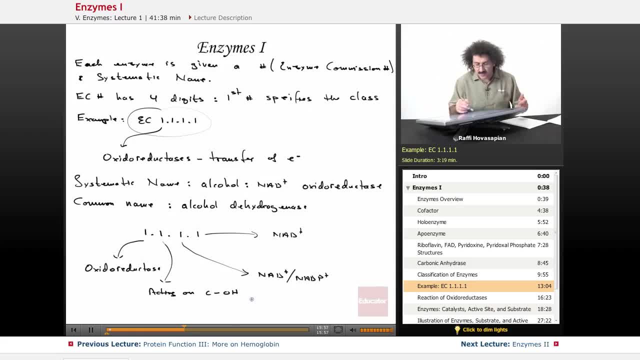 The sixth one is NADP plus, The seventh one is NADP plus And the last one is NADP plus. That's it So really, what's I mean ultimately? what's important, I mean, are all of the numbers. 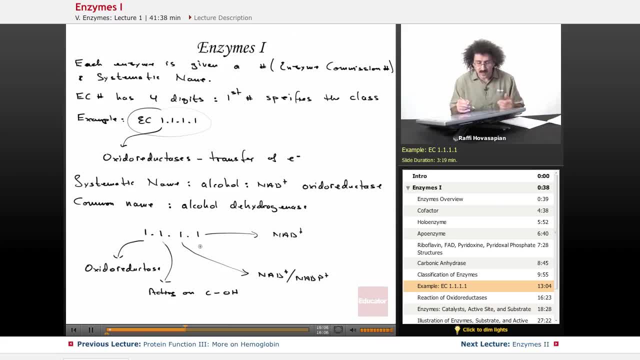 I mean, you can look all of these up, It's not a problem, You don't have to know any of these. It's really important to know that. the first one is what specifies the class And your teacher will probably ask you to know. at least you know that. 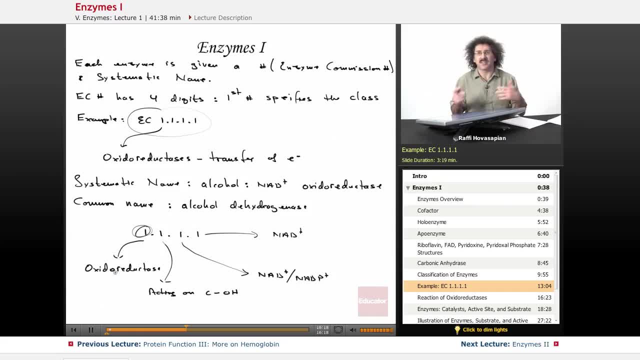 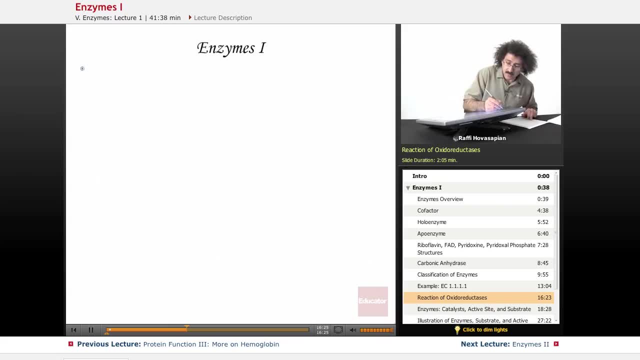 The six classes of. so you have oxidoreductase, you have lyase, you have ligase, things like that. So that's all that's going on here. The particular reaction that this enzyme catalyzes is the following: 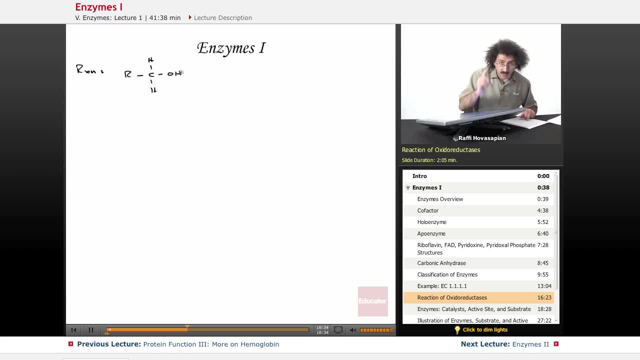 See, it takes a primary alcohol, primary alcohol. So the enzyme binds two things: It binds the alcohol and it binds the NAD. plus, It brings them in close proximity and it allows the transfer of electrons and hydrogen from this, from the alcohol, to the NADH- I'm sorry, to the NADH. 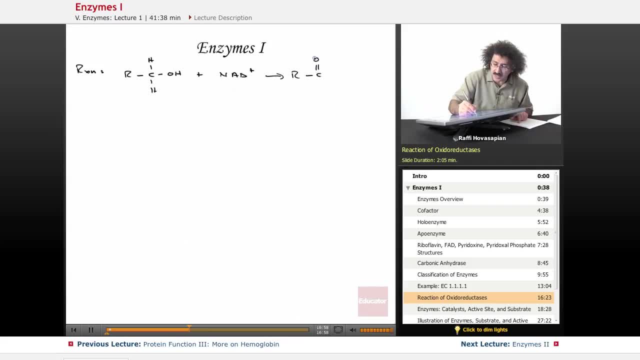 NAD plus to produce the following: What the enzyme ends up releasing? you end up turning the alcohol into an aldehyde, And then you've also created this thing. That's it. That's it Basically. all you've done is you've what this enzyme done is: it rips away that hydrogen. 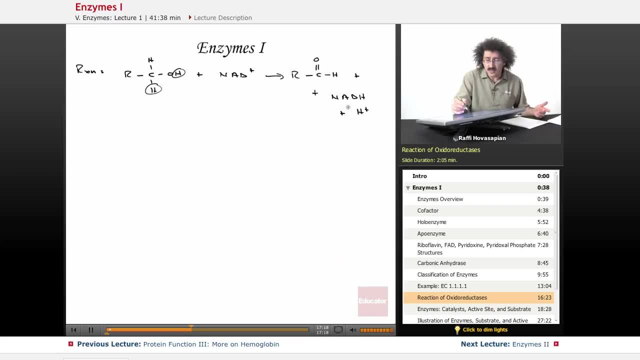 that hydrogen. It turns this single bonded oxygen into a carbonyl And then it releases something called NADH and H plus into solution. Okay, Okay, So alcohol dehydrogenase. Now, of course, you probably already know this. 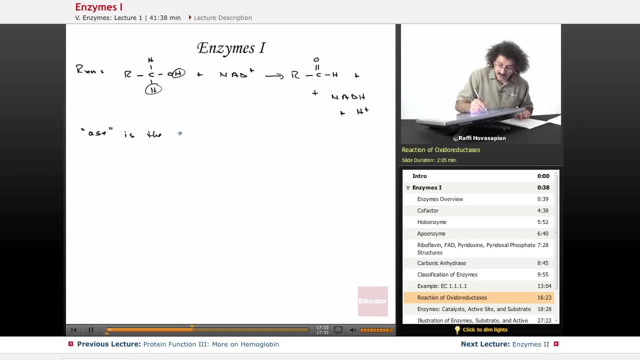 If not, ACE is the standard ending, standard ending for an enzyme, For an enzyme. So alcohol dehydrogenase, pyruvate dehydrogenase, something, isomerase, hexokinase, ACE-ase. Okay, That's ACE-ACE-ACE. 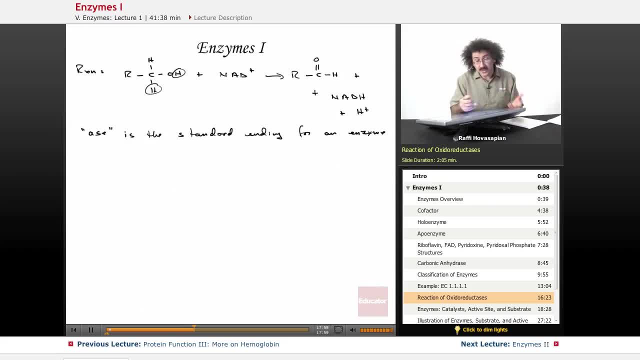 That's the enzyme, In this particular case, the cofactor. this enzyme does have a cofactor. The cofactor happens to be that molecule, So- and in this particular case it's a cofactor that is not tightly bound to the alcohol dehydrogenase. It's actually free to float around. So we don't call it a prosthetic group, but we do call it a coenzyme. Okay Now, Enzymes are catalysts. Okay, Let's go to blue here. So enzymes are catalysts. 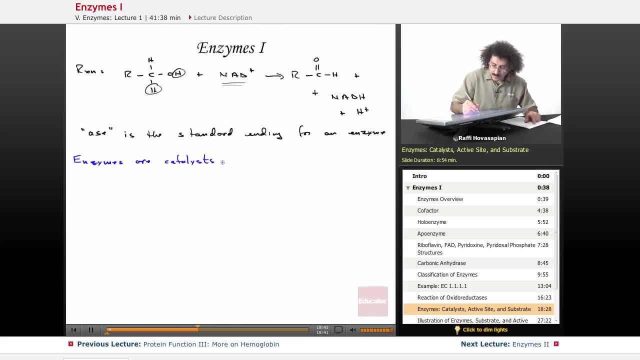 That's it. They're just, they're- catalysts. All they do is they speed up a reaction. They speed up a reaction, Okay, Okay. So they do not, but do not, they do not affect the equilibrium position of a reaction. 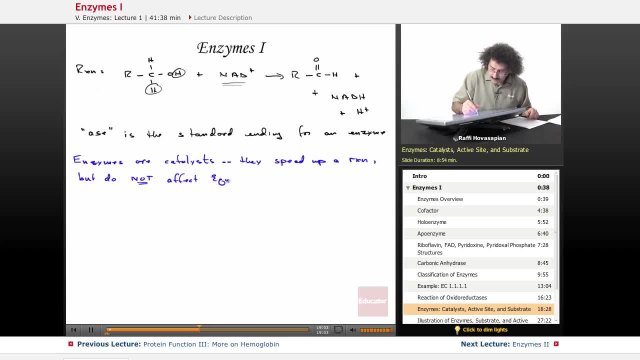 That's very important. They allow a system to come to equilibrium faster. they just don't change the equilibrium position. So again, there are many reactions that can take place. For example, if I want toif I put oxygen and hydrogen in a container. 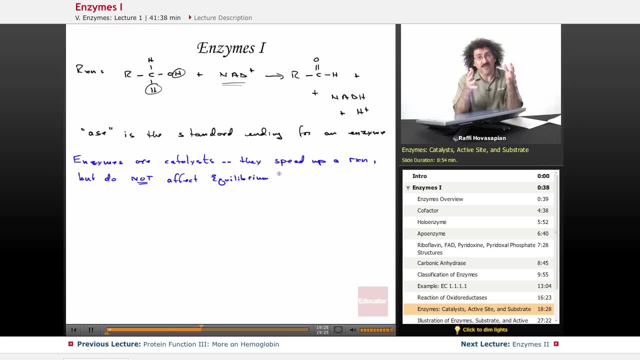 container. Well, thermodynamically that reaction wants to happen. It's very thermodynamically favorable. The problem is: kinetically it's not. because it has a very high activation energy. It takes a lot for it to go over that initial hump in order to become water. So thermodynamics and kinetics are not the same thing. A catalyst does not affect the equilibrium. It affects how fast it reaches equilibrium. That's it. That's all a catalyst does, So it just speeds things up. Now, under physiological conditions- bioreactions- they tend not to. 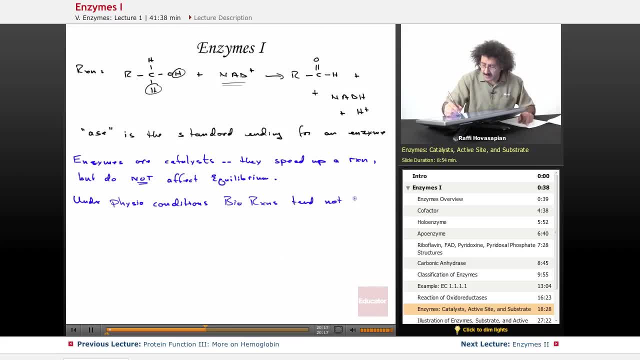 happen. In other words, they're not too thermodynamically favorable. They tend to happen, or they happen very slowly. Again, this is why enzymes evolved. They evolved to allow for life processes to function without having to wait forever. It's really kind of. 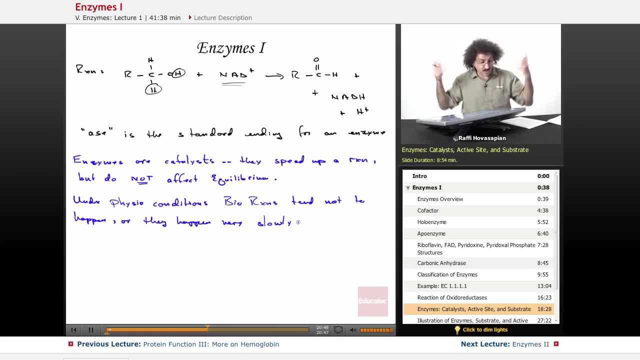 amazing, Many of the reactions that give rise to life, like you know, like you know, you know life shouldn't happen, wouldn't happen. Enzymes allow them to happen. Absolutely extraordinary, powerful, powerful things. It's a lot more than just speeding up a reaction. It's the 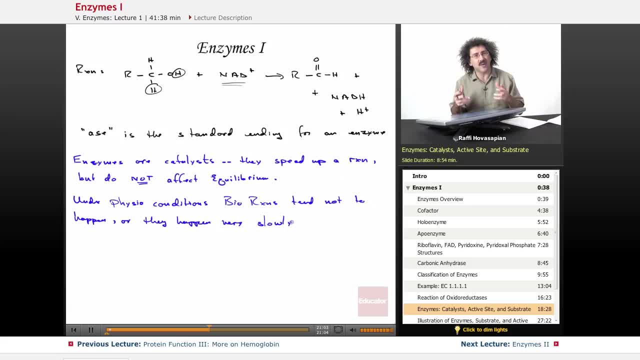 extent to which they actually allow reactions that are so complex to actually take place, Reactions that would never happen in the body, but enzymes allow them to happen. So okay, Now it does this. It does this, in other words, allow the reactions to happen by providing, providing a place. 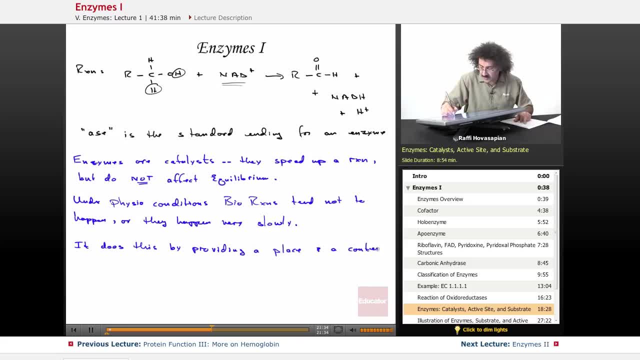 an actual physical place and a context, an environment for the reaction to take place. We call this place the active site, Very, very important. So where a particular something happens in the enzyme is called the active site. It's where the reaction takes place. 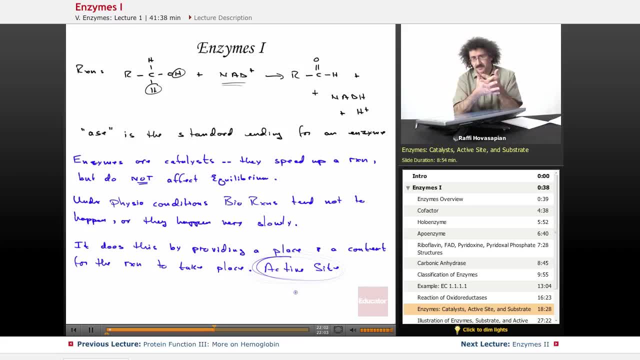 Now I want you to think about this. You've got a whole bunch of. you've got just just billions and just millions, thousands, whatever different types of molecules floating around in your body in any given space In order for a reaction to take place. well, a couple. 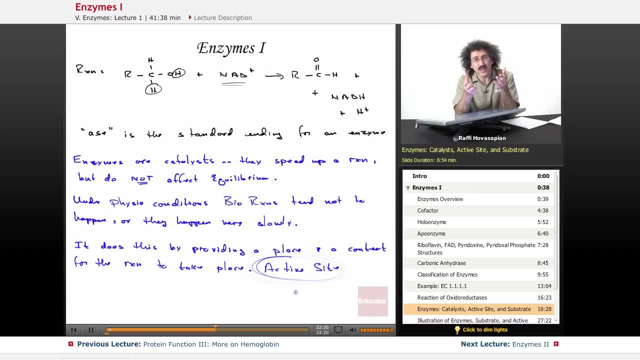 of things need to happen, The most fundamental of which is that, let's say, if you have to have this molecule, react with this molecule. Well, it's like being in a hugely crowded city. How is it that one molecule on one side of the city is supposed to run into one molecule in the other side? 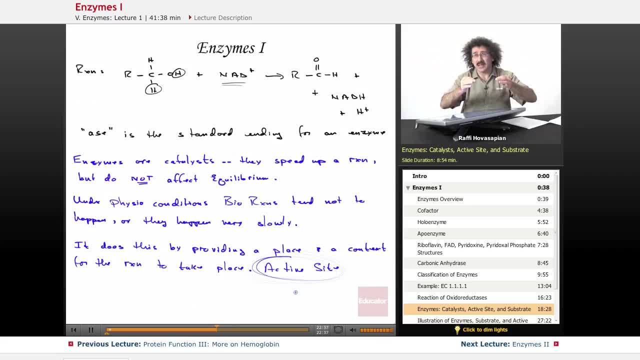 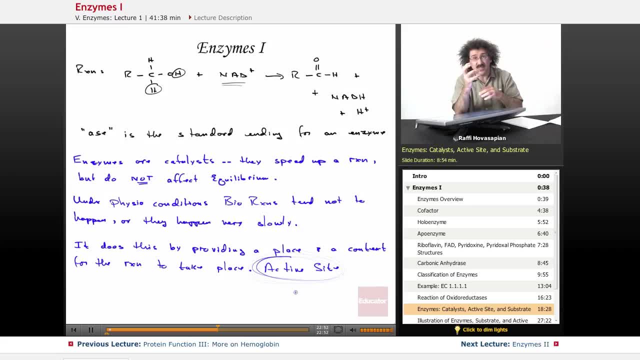 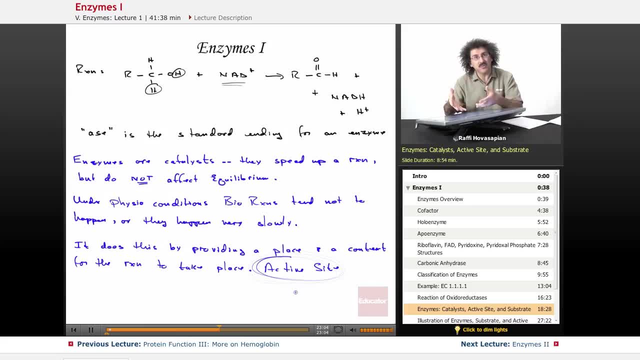 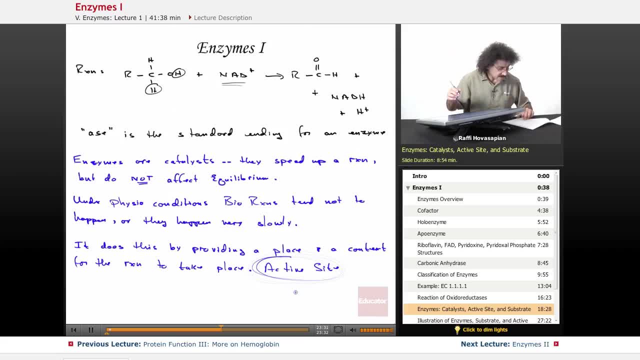 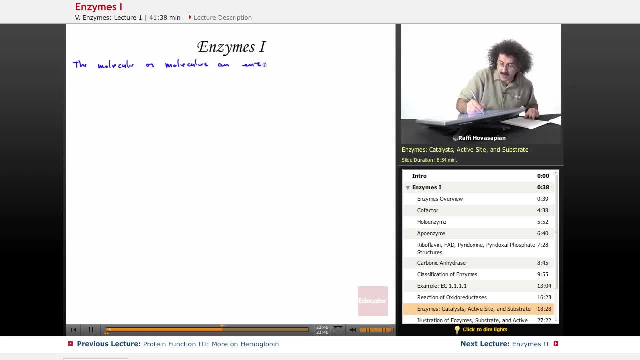 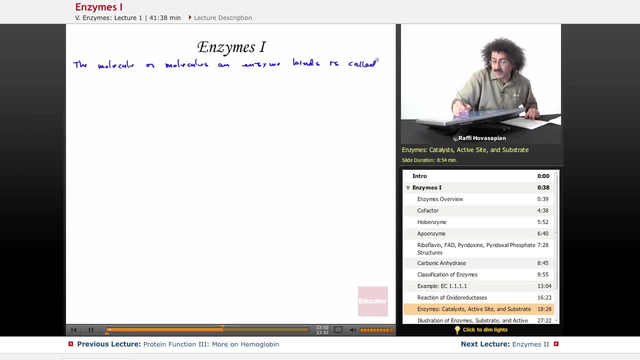 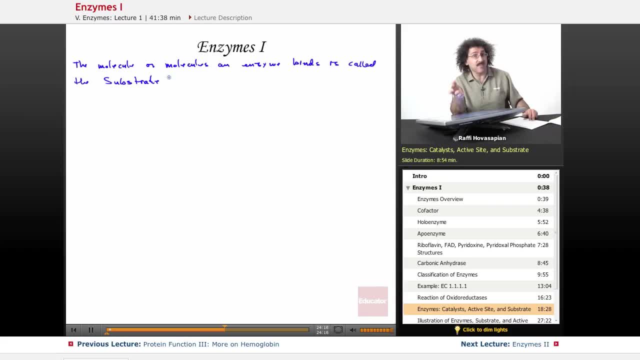 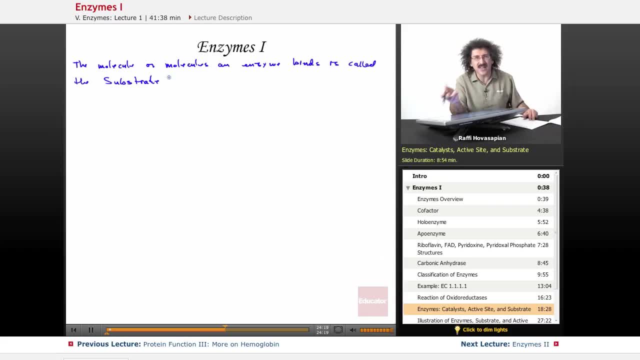 also a substrate. It's the second substrate. Again, a lot of these things happen more to do with names. Names are not altogether important. What's important is what's happening. In this case, it brings together the alcohol and the NAD+ in order for them to do what they need. 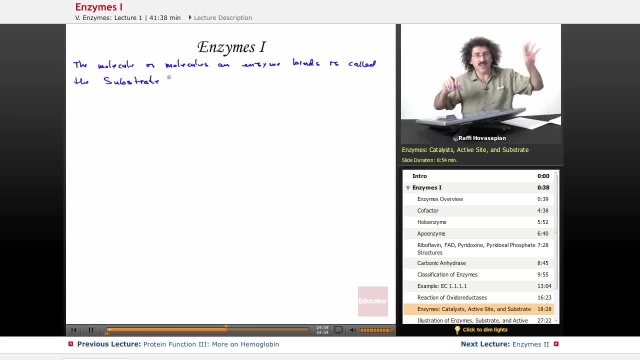 to do, then it sends them off on their way. The alcohol leaves as aldehyde, the NAD-plus leaves as NADH and the enzyme goes and does it for another pair of molecules. Molecular molecules and enzyme binds is called the substrate, The active site. you guys already 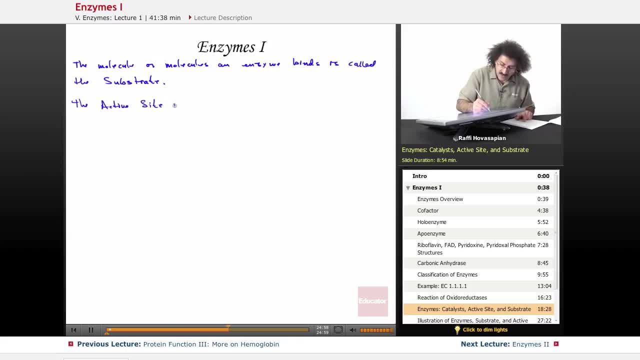 have a sense, I think, of what enzymes are. The active site is often a pocket on or within the enzyme- Okay. And because an enzyme is a protein, this pocket is lined with amino acids which bind the substrate. Okay, They bind the substrate with weak interactions. Basically, you have this pocket and along 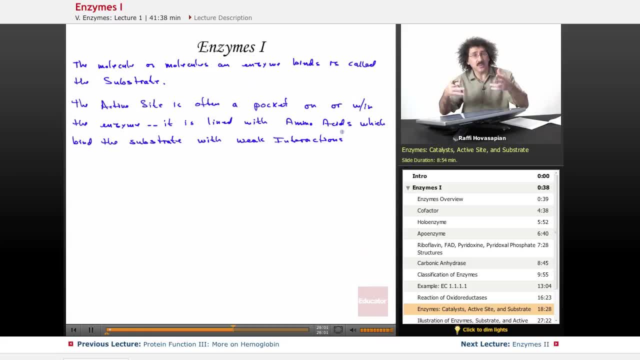 the pocket. there are these amino acids which are part of the protein, part of the enzyme. They interact with a substrate in certain ways, with weak interactions, hydrogen bonding, ion dipole, hydrophobic interactions. They sort of form a little bit of a cocoon, a little support for the particular substrate, and then it 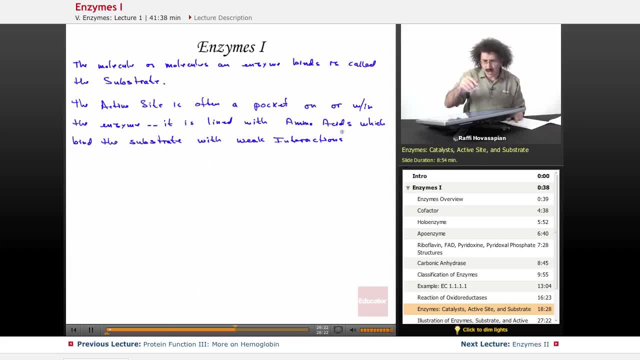 allows it to do whatever it does. We'll be talking a little bit more specifically about binding and weak interactions and things like that. Okay, So amino acids which bind the substrate with weak interactions- Okay, Often the substrate Okay. 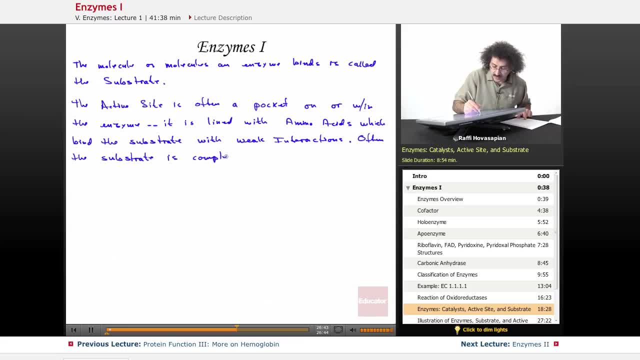 is completely sequestered from solution. It's completely sequestered from the environment, From the aqueous environment. So, in other words, when the enzyme binds the substrate, it doesn't allow water or anything else to come in. Okay, There's no space for only that molecule and whatever else needs to be there for the reaction to take place. So that's what we call sequestering: It separates it from solution, so you don't have a bunch of other stuff floating around. 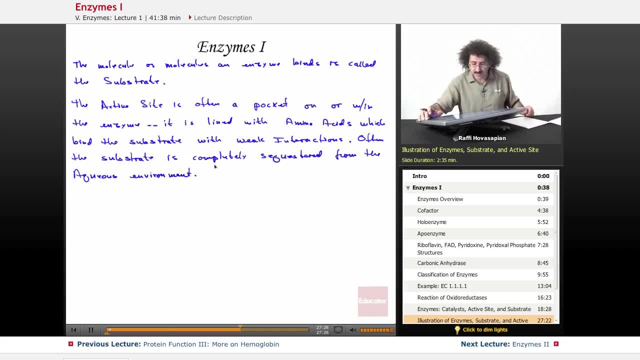 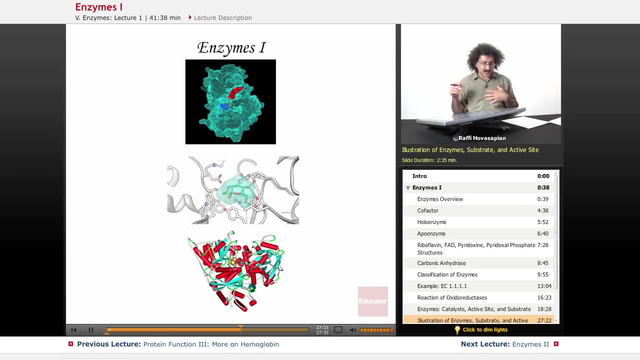 So let's go ahead and just take a look at some of these things just to get a sense of what they might look like. So let's see, Here we have an image of three dihydroquinate synthase. In this particular case, we have three synthases. 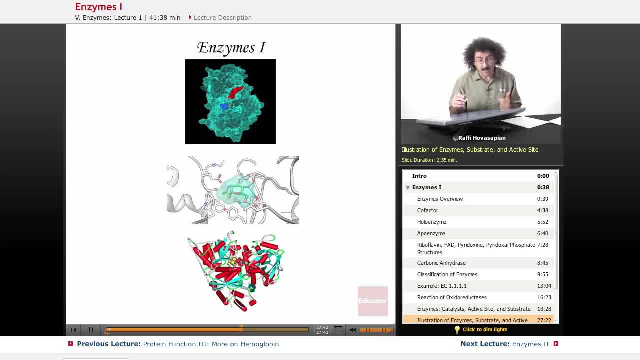 We have three substrates. We have three things that are attached. Some of the substrates are cofactors, Some of them are not, Again, just things that are attached to it. We have here, if you can see it, this thing is zinc. 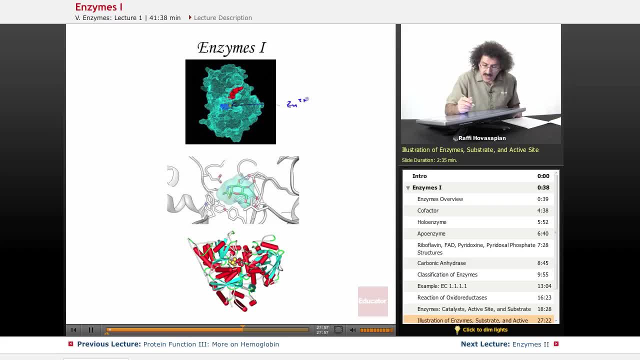 It's a zinc ion, And over here we have another substrate that looks like it's going to be the NAD+, And over here is the other substrate, the actual substrate itself. It's something called carbophosphonate. Okay, 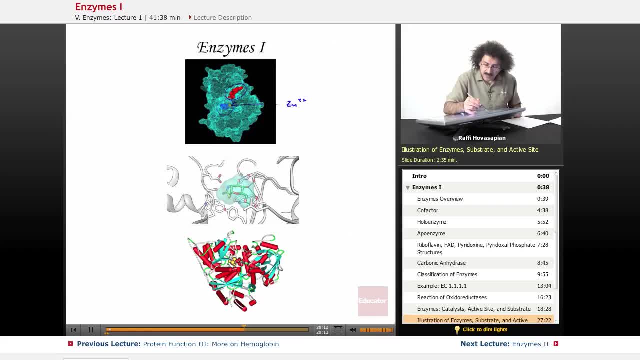 And again you notice on here, this is a sort of a surface image of the enzyme. You notice that this particular binding pocket happens to be on the surface, This one, the substrate, seems to be actually inside, So it's a pocket inside of it. 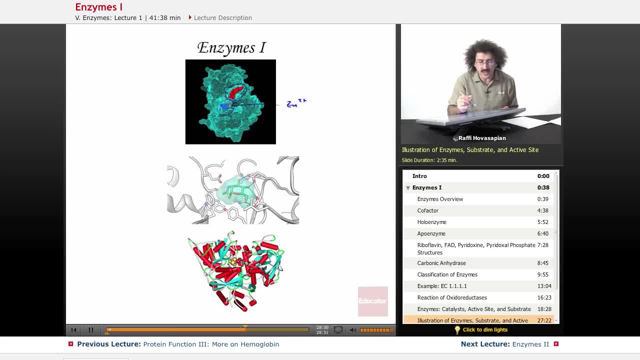 The enzyme has sort of closed itself around it. So it's not necessarily on the surface and it looks like the zinc is on the inside too. Here the second image. It sort of shows a close-up of a substrate which is this thing right here and some of. 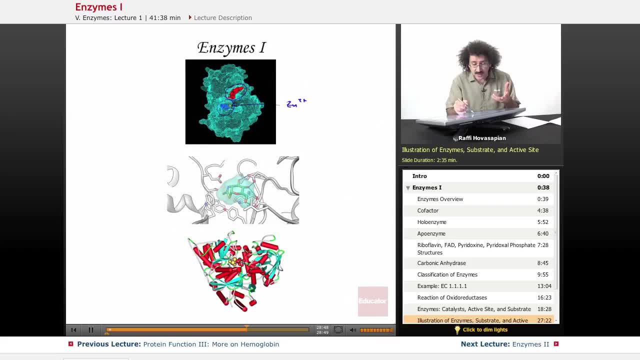 its interactions with the amino acid residues that make up the active site. So here you can see that here's oxygen, oxygen on here. I don't know which molecule this is, but it looks like it's interacting a little bit with this thing right here. 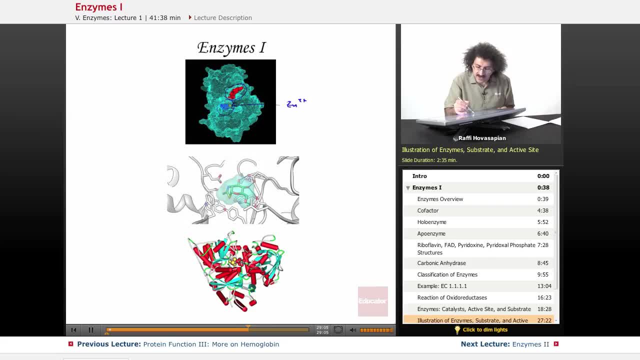 You know, it looks like maybe a carboxyl group, maybe a glutamate, something like that, And notice this is attached to the protein. So this is the protein, the amino acid side chain. It's the amino acid side chain that's actually interacting with weak interactions with the 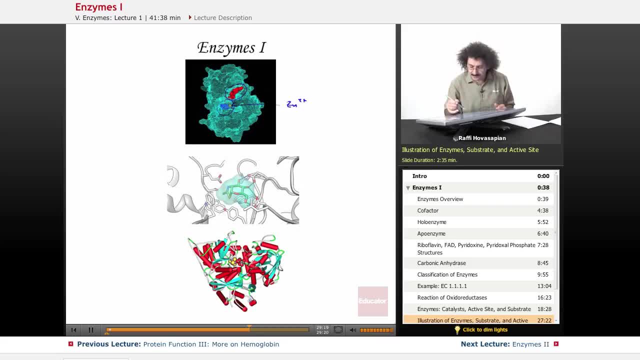 particular substrate, And that's it And another sort of- you know another view of it. Here we have sort of a surface image. Here we have a ribbon diagram. Again, you can see the substrate is actually right here and it looks like it's actually. 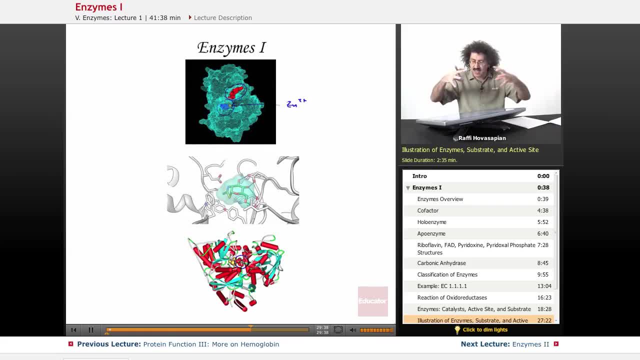 deep inside of this particular enzyme. It looks like maybe the enzyme opened up, substrate came in and it closed itself around it. That often happens. We'll be talking about that a little bit later too. something called induced fit, That's it. 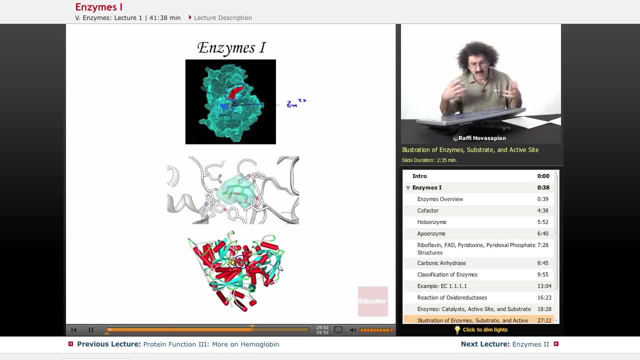 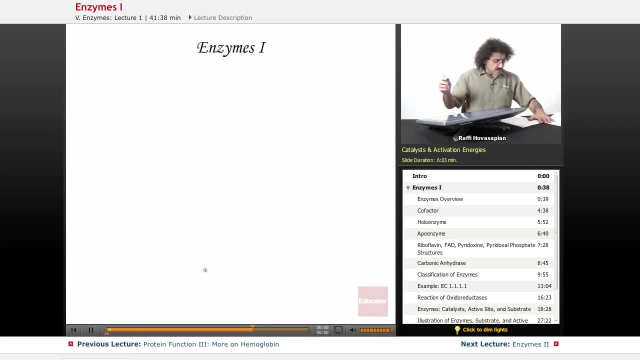 That's all it is. Active site enzyme, sometimes on the surface, sometimes inside the enzyme. nothing particularly strange going on, Okay, So let's talk a little bit about how catalysts do what they do. So catalysts Okay. 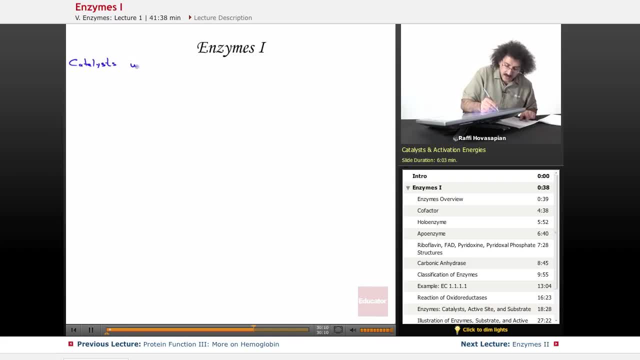 So catalysts work by lowering activation energies, That's it. You know from general chemistry that that's what catalysts do: Activation energies, and or providing an alternate pathway, I don't know. Okay, The thing is, by providing an alternate pathway, you're lowering the activation energy. 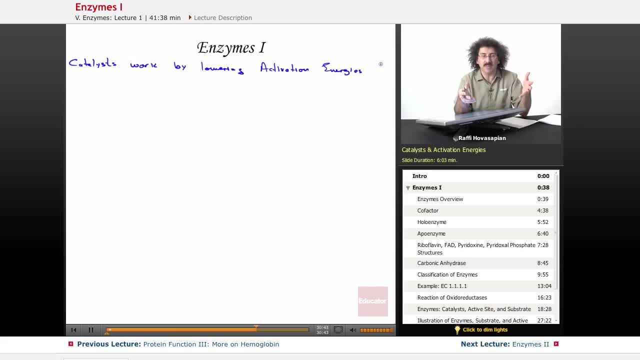 So shall we say lowering the activation energy and or providing an alternate pathway. Let's just say, catalysts work by lowering activation energies, How's that? And Let's just say: and Providing alternate pathways, Alternate pathways for the reaction to proceed. 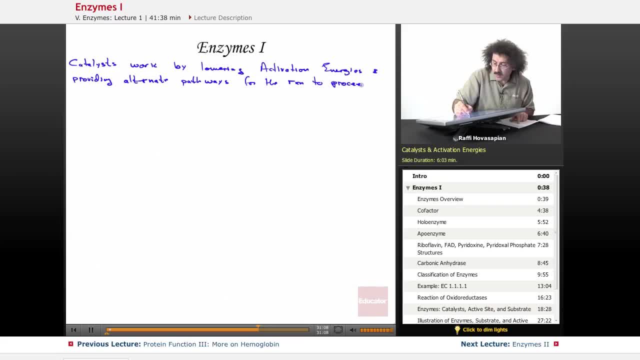 Okay, So in terms of an energy diagram, let's take a look here. So we might have that and we might have that, Something like this. So this is our substrate or reactant. Let's just go ahead and call it a substrate from now on, because we want to get used to. 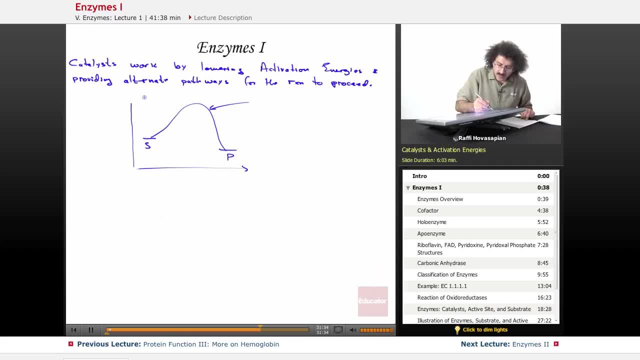 this nomenclature And this is going to be the product. So this difference right here, The difference between here and here, This is something called the activation energy. This is an energy hump that the substrate has to get over before it's in a position. 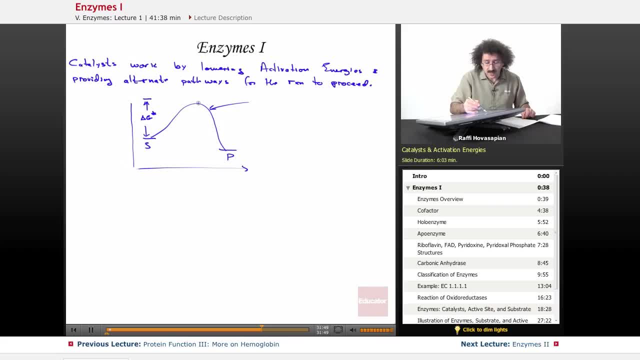 to actually fall forward and move on to product. And this right here, This is called the transition state. So it has to reach the. well you know what? let me do this in red. So this right here, Okay, This has to reach the transition state. 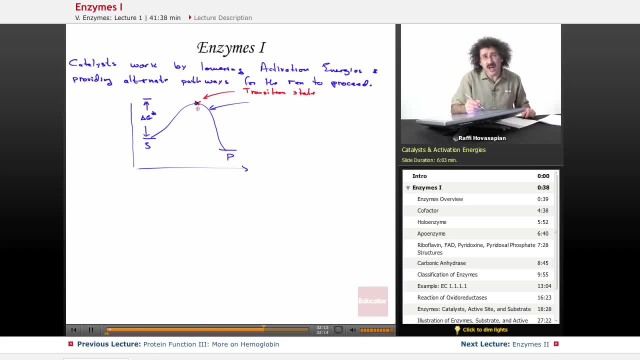 And often this energy barrier, this activation energy, is very, very high. This energy barrier is what controls the rate of the reaction. The lower that energy barrier, the faster the reaction is going to go, because more molecules are going to have enough energy to get over that hump. 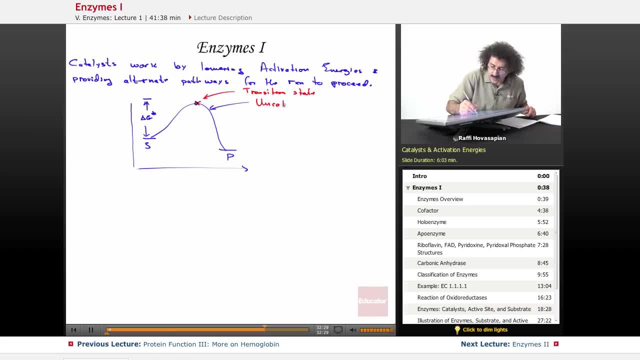 So this right here, this path, this is the uncatalyzed reaction. Okay, This difference right here, The difference in energy from here to here. This is the normal delta G. That's the thermodynamics of that. Now the catalyzed reaction might go something like this: 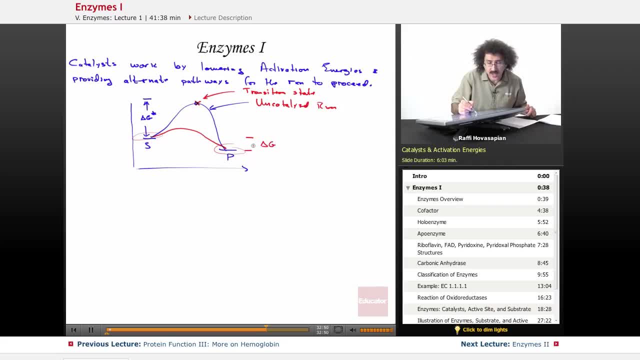 So notice this and this haven't changed. We're still here and here. The delta G hasn't changed. Thermodynamics doesn't change. What has changed is this: Now, your activation energy is a lot lower. Because the energy is a lot lower, the reaction can proceed faster. 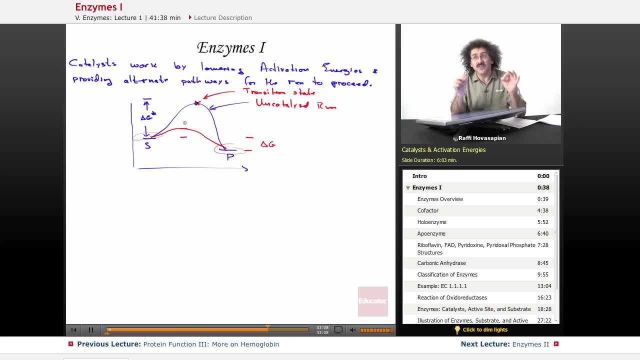 That's what a catalyst does. That's all a catalyst does. It is not used up in the reaction. A catalyst itself. it goes in in one form. it comes out of the reaction in the same form. In between it might experience some changes, but itself has never changed from beginning. 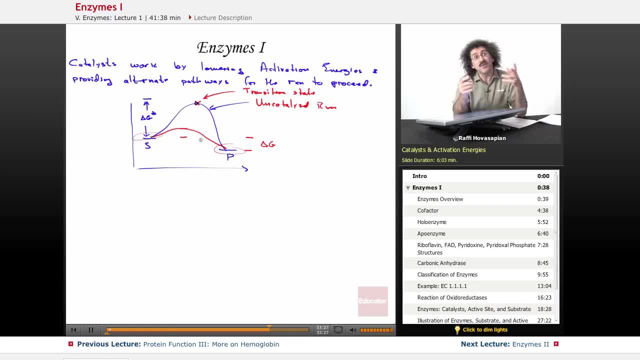 to end of the reaction. All it does is it provides a different pathway for the reaction to proceed. That's all. That's how a catalyst does what it does by reducing the activation energy, the energy it takes to get over the transition state. 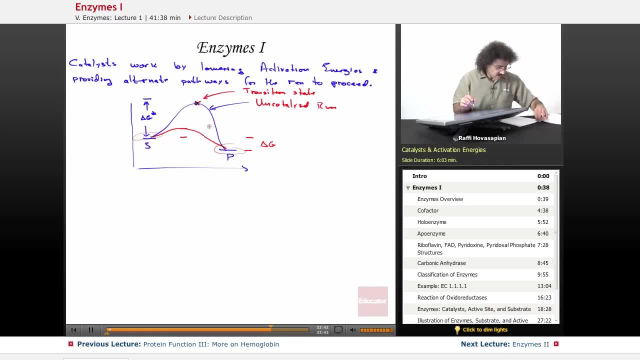 Now let's go ahead and see, Let's do one more energy diagram here. This is substrate, This is product. Let's go ahead and make that here. Actually, you know what? Let me go ahead and since I used blue for the uncatalyzed, I'll go. 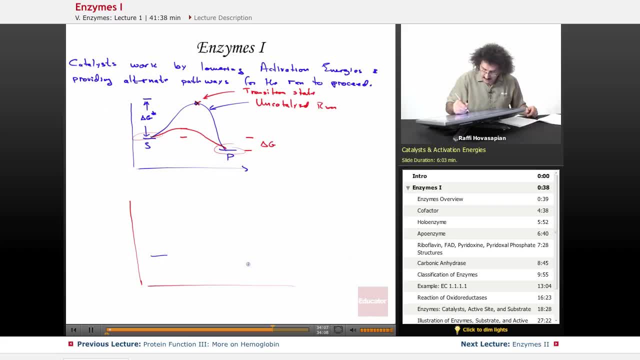 ahead and keep it as blue for the uncatalyzed Here, here like that, and we might have something like this, Something like this. So here what we have is we have enzyme plus substrate. It's going to form something called the enzyme-substrate complex. 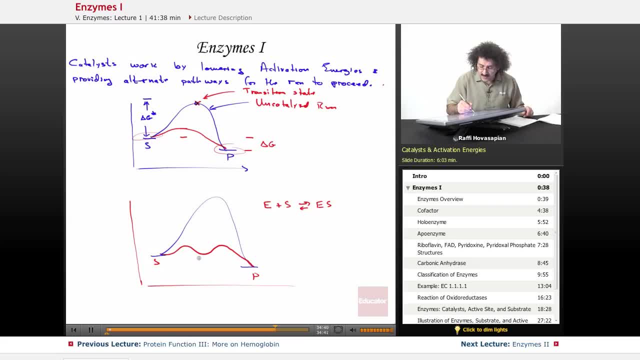 Once the substrate binds to the enzyme. now we have this thing. Actually, you know what? Let me, I think I'm going to do two hills, because I need two hills, And then we'll go there. How's that? So here, this is our enzyme. 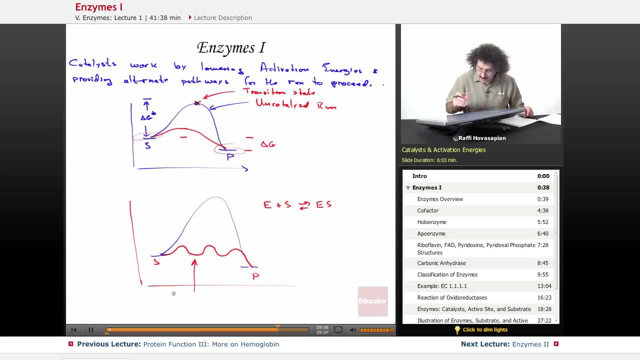 This is our enzyme-substrate, Enzyme-substrate, And here we have our enzyme-product, Enzyme-product, And of course the enzyme is released and the product is released. So the enzyme and substrate come together. They form something called the enzyme-substrate complex. 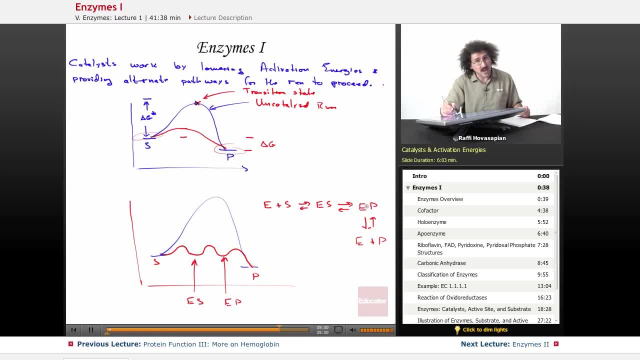 The substrate is converted, changed to product. Now we have the enzyme-product complex And then the enzyme and product separate. The product is released and enzyme goes back to start a new cycle. It can be represented like this: The substrate starts here. 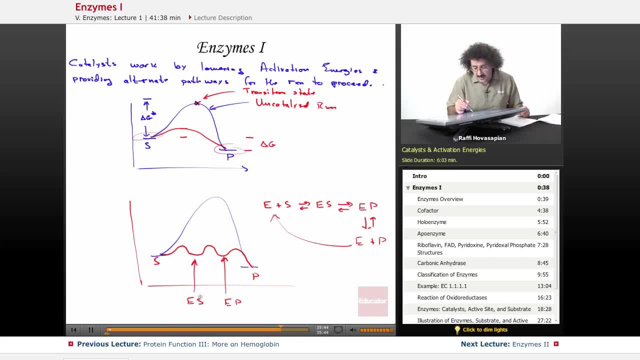 This first hump in order to get to this first intermediate. this intermediate is the enzyme-substrate complex, And then it goes to the next hump- enzyme-product complex- And then the next hump in order to actually release this. 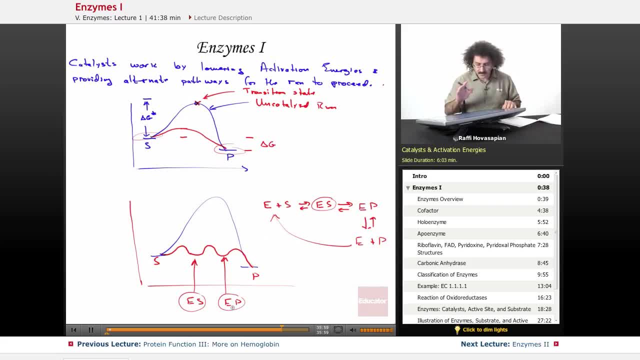 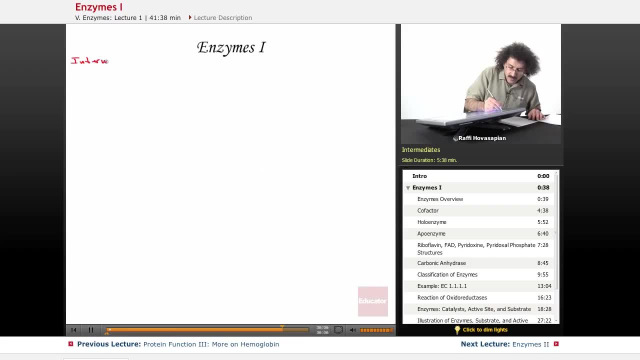 So here, well, I'll tell you what. Let's look at this, Let's look at this, Let's look at this, Let's go ahead and just talk about it. So intermediates are short-lived viable species in a reaction pathway. 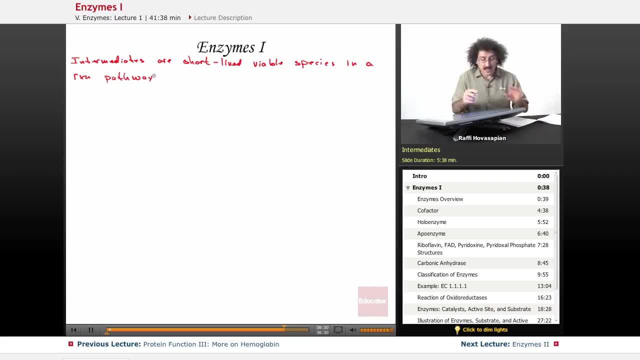 Now, in this case, by pathway I mean individual reaction in a you know what- I won't say pathway, because we're going to actually use pathway in a different context. Intermediates are short-lived viable species. I'll say in the progress of a reaction. 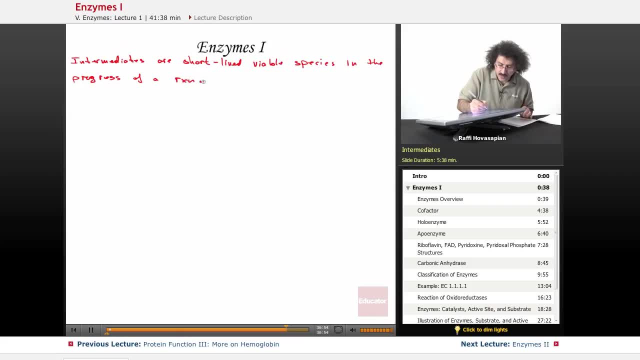 In the progress of a reaction. So, in other words, it isn't just reactions don't necessarily happen in a single step, They happen in multiple steps for a given reaction. Each one of those steps has a little transition state that you have to get over. 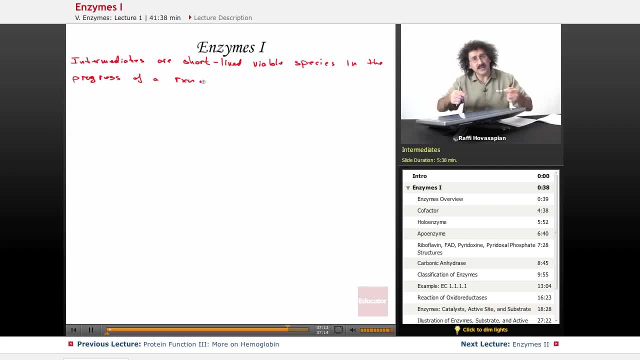 And each one of those valleys constitutes an intermediate. So an intermediate is something that is there. It is short-lived, It doesn't live very long. So in the case of an enzyme to an enzyme-substrate, it has to go over a small hill to become an 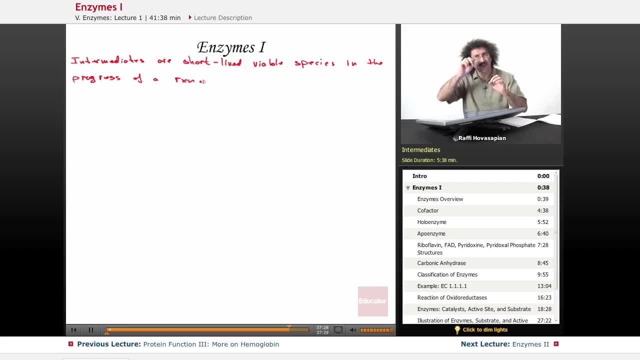 enzyme-substrate. Now, that's an intermediate. Now the enzyme-substrate has to go over another little bump to become the enzyme-product, And then the next bump in order to actually become the product. So again, we have to differentiate between intermediate and transition state. 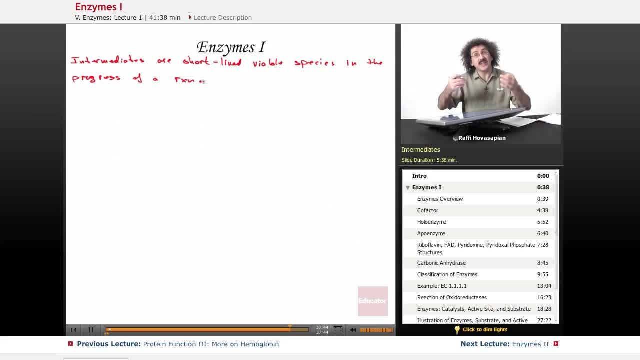 They're not the same thing. A transition state is a very small fleeting thing that the particular substrate has to pass through in order to become the next thing. So an intermediate is a place along the way from substrate to final product, sort of you call it an intermediate. 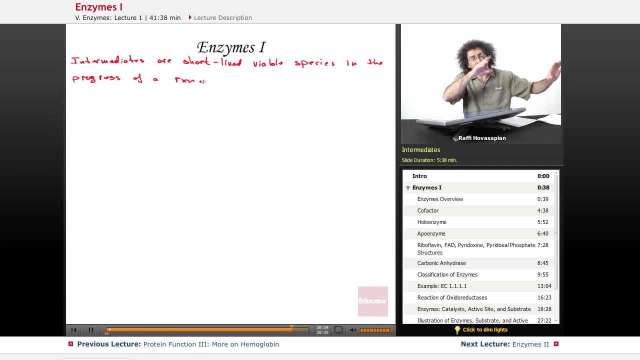 Intermediate product, if you will. It's something that it has to pass through. It's a low-energy point, not a high-energy point. Okay now conversion from one intermediate to the next intermediate. So if you look at the reaction steps, the slowest of those steps constitutes a reaction. 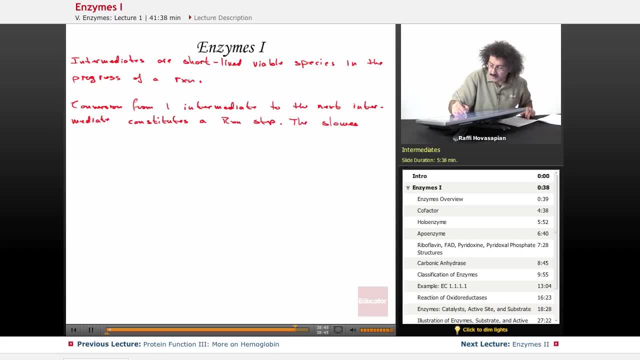 step That constitutes a reaction step. The slowest of those steps is called the rate-limiting steps. So if a reaction takes place in five steps and one of those reactions is actually the slowest, that's the rate-limiting step. 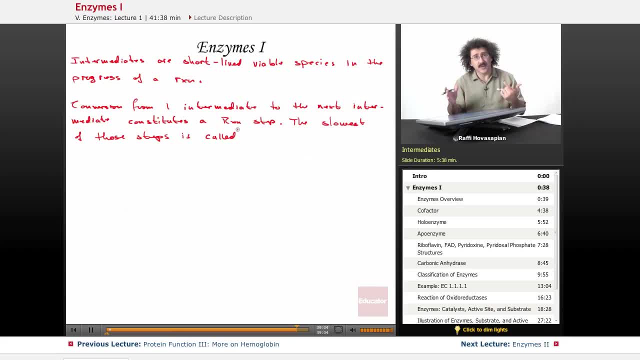 And that slow reaction is going to control the overall rate of the reaction, because you can only go as fast as your slowest step. That's it. A chain is only as strong as its weakest link. The slowest of those steps is called rate-limiting. 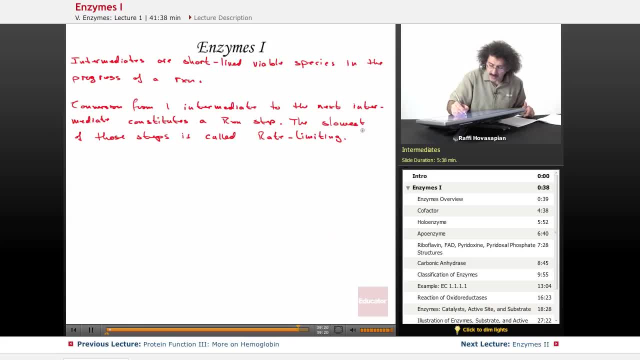 Makes perfect sense. Nothing strange here, Completely intuitive. Now here we're talking about individual reactions that happen in multiple steps. So if you look at the rate-limiting step, you can see that the slowest of those steps is called the rate-limiting step. 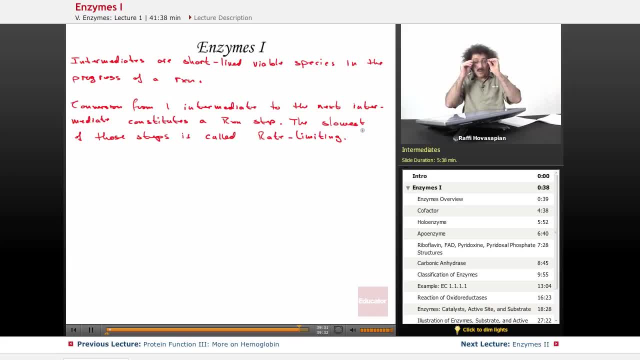 That's the rate-limiting step. That's the rate-limiting step And again, we're only going to be talking about individual reactions that happen in multiple steps, Most of what we discuss when we start discussing the metabolic pathways in the second half.